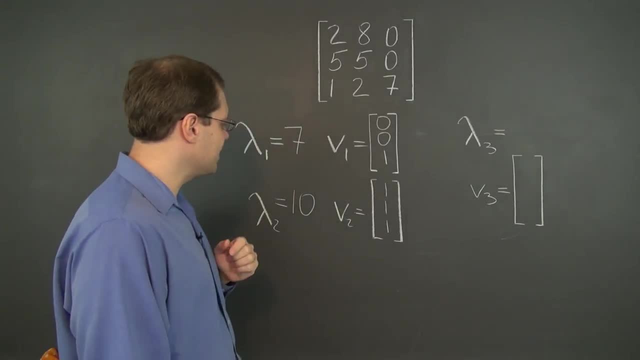 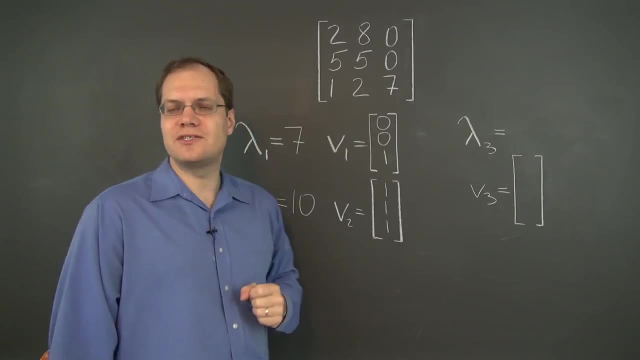 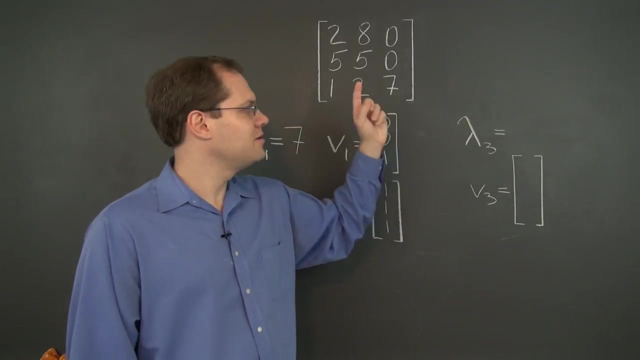 will tell us the third. these two eigenvalues add up to 17 and all of them together add up to the trace of this matrix, which is 14. so this one must be minus 3, so that 7 plus 10 minus 3 is the trace. 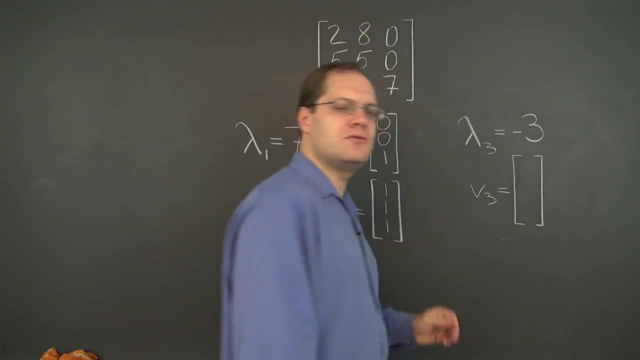 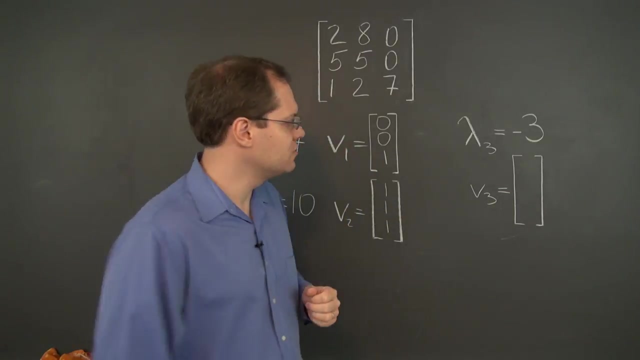 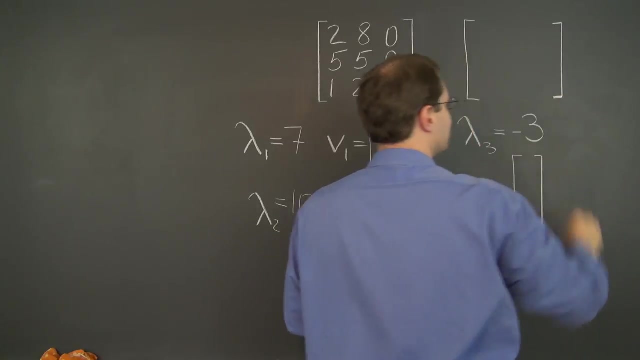 so this one is minus 3 and we do not know from the trace alone the corresponding eigenvector. so we still have a little bit of work to do, and I'll do it right here, although we've done it several times before. I think it's kind of magical how this works out, because I think that the trace 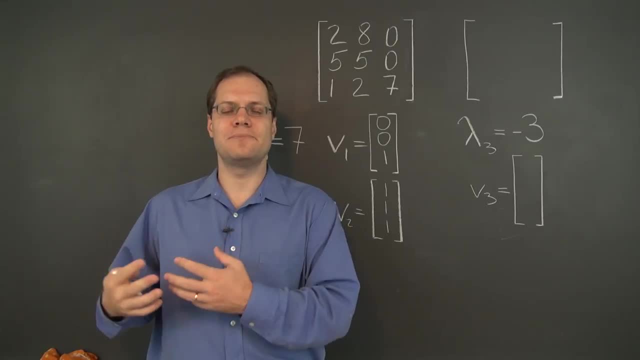 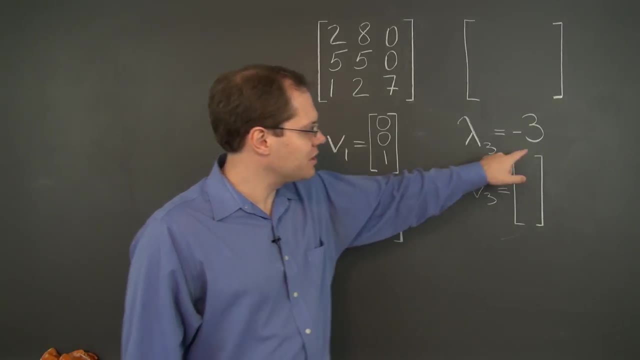 property. adding up to all of the eigenvalues, even though it's simple to prove, is a magical sort of thing. so it's kind of amazing how we did almost no work at all and we can be completely sure that this is an eigenvalue of the matrix, even though by just 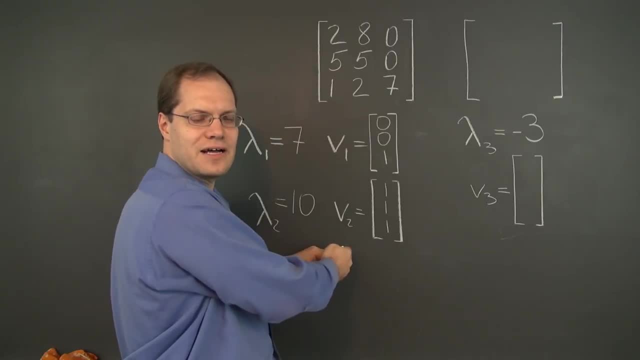 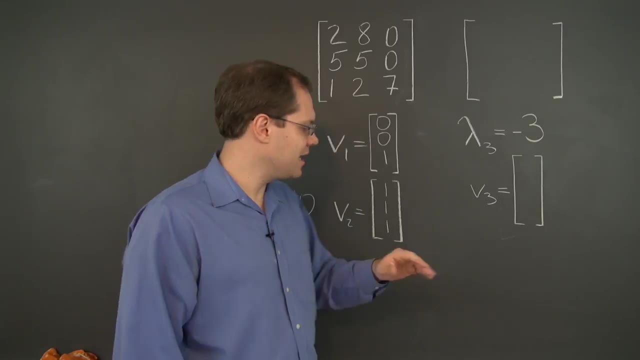 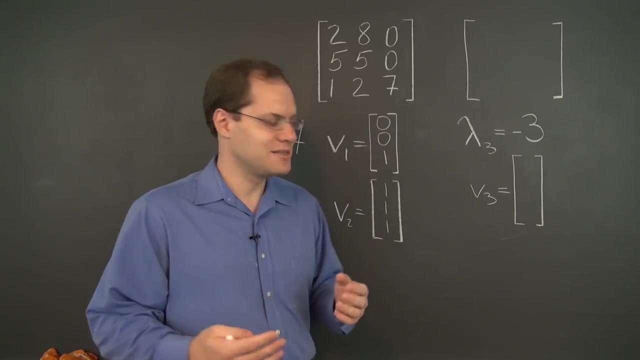 looking at the matrix without identifying the other eigenvalues. there is no evidence whatsoever that would suggest that negative 3 is an eigenvalue. so we kind of knew that minus 3 is an eigenvalue from other considerations, rather sophisticated considerations and a variety of different features that we took advantage of. so I still think it's magical. 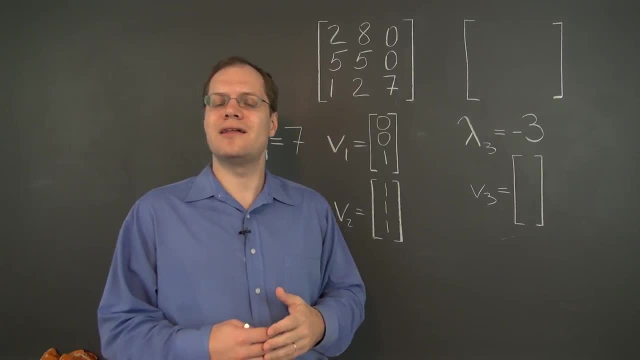 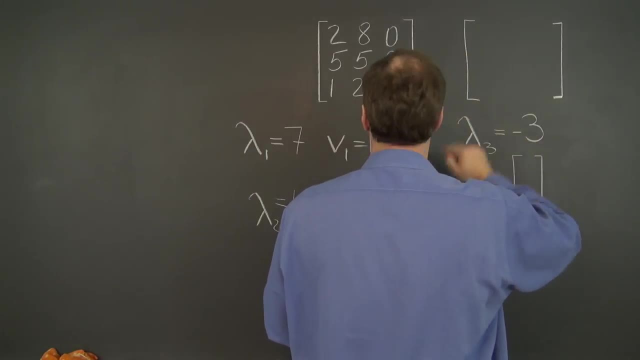 to sort of figure out how to do this, and I'll see you in the next video. subtract minus 3 from the diagonal and realize that, lo and behold, we have a singular matrix. so subtracting 3 is the same, subtracting negative 3 is the same as adding 3. so we're left with 5, 8, 10. 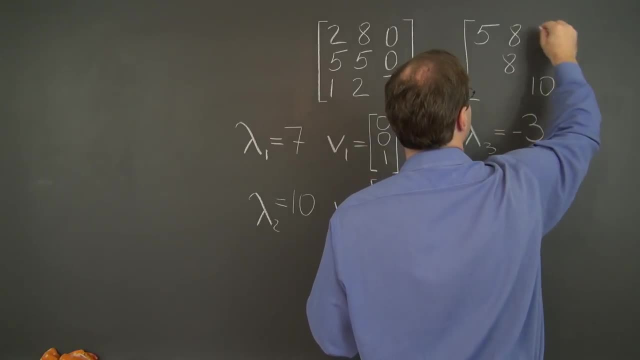 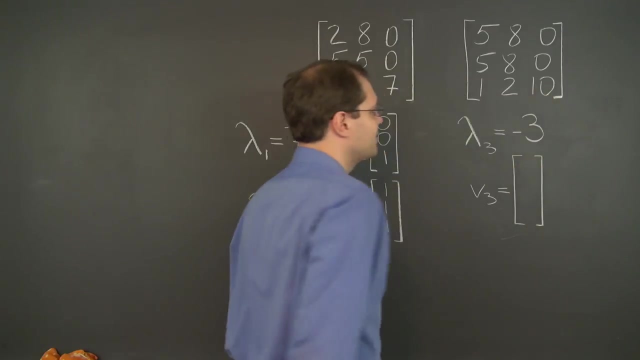 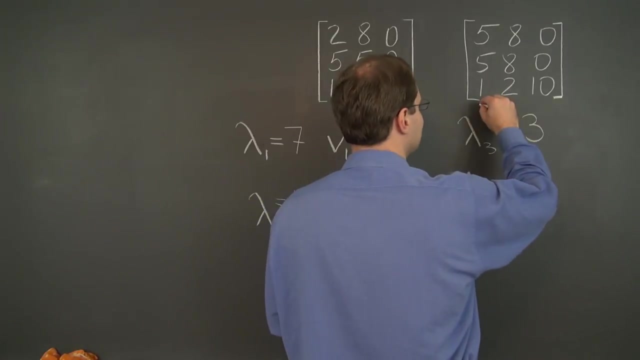 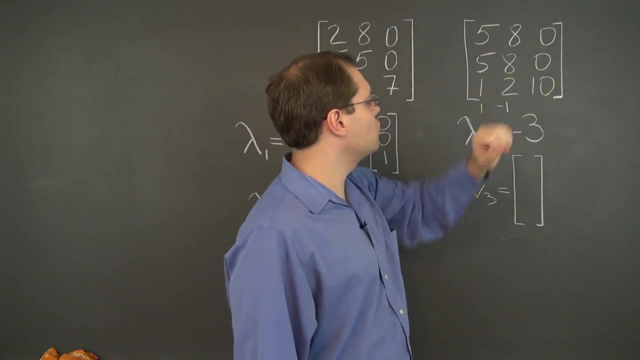 all right. and the remaining entries are the same: 8, 0, 5, 0, 1, 2. all right, and indeed we have a singular matrix, a very satisfying feeling, and of course, we need to take these columns in proportion, 1 negative, 1- so that the first two- oh no, what am I saying? we have to take the first two. 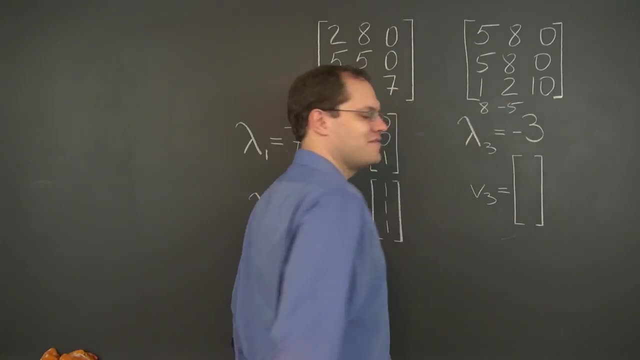 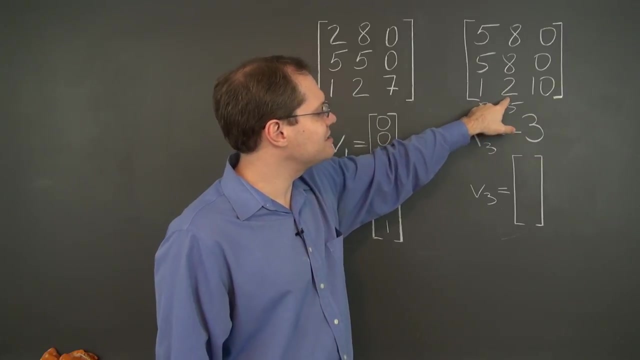 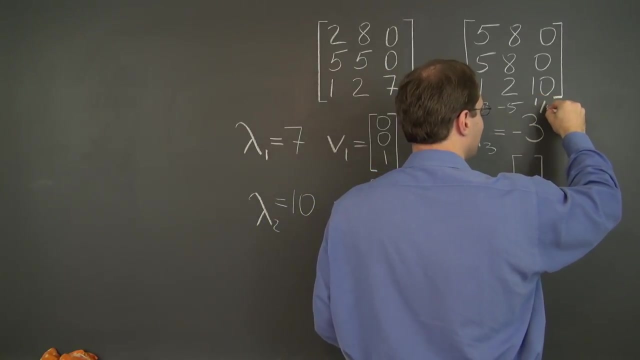 columns in proportion: 8 negative 5, so that the first two entries cancel. and then in this entry we have 8 minus 10. 8 minus 10, that's negative 2. so we have to take 1, 5th of this one. let's just make.